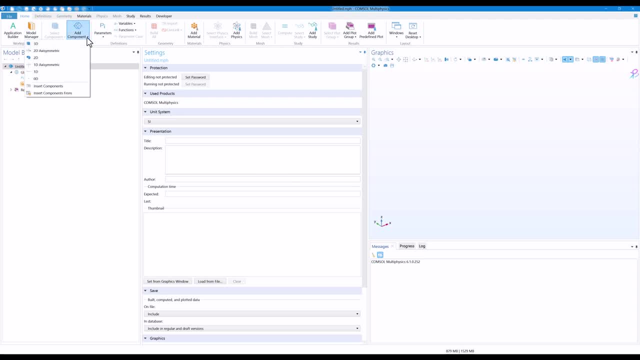 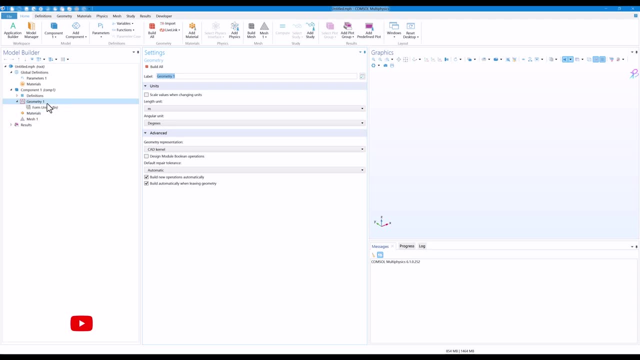 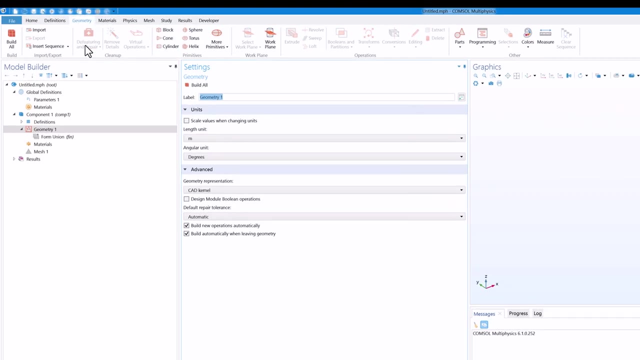 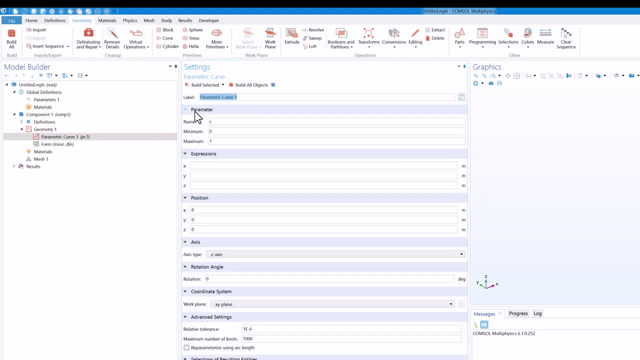 in the home tab, click on add component and then 3d component. so at first we'll have the geometry. now we'll go on to geometry, and at first what we will do is that we'll click on more primitives and then click on parametric curve. now in the parametric curve we will write: 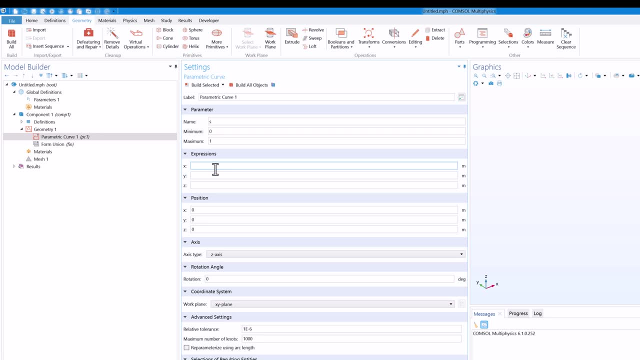 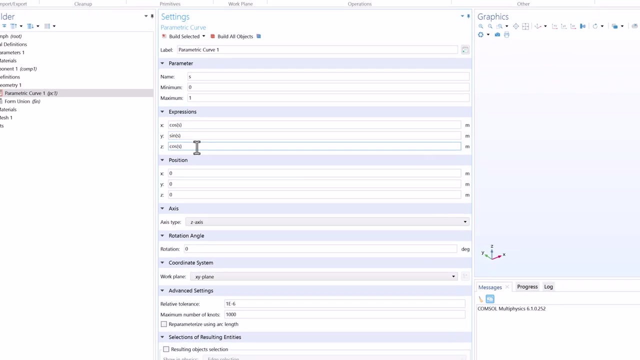 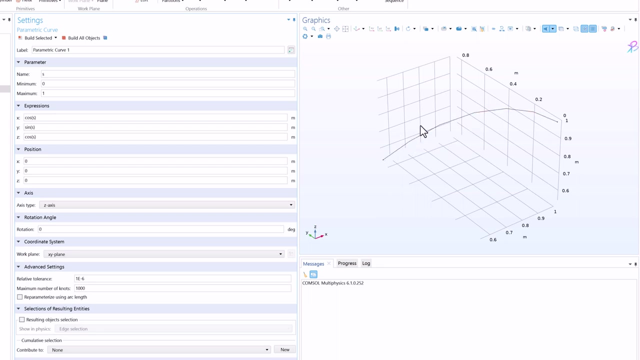 expressions to create curve. for example, if I write cos of s- and here I will write sine of s and here again let's say cos of s, and if we click here, then you will see that we will have a parametric curve and the x, y and z coordinates. 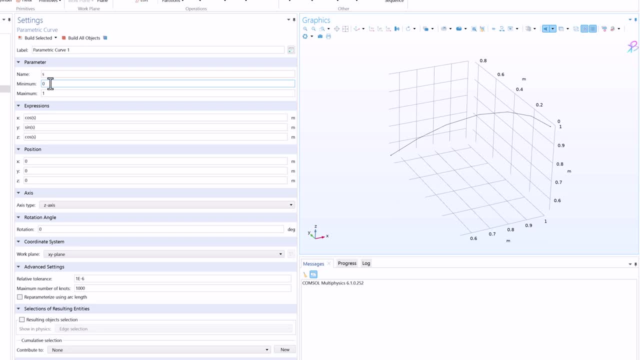 are given by this expression, where the value runs from 0 to 1 and the s is evaluated for x, y and z. so this is how you create parametric curve. now, of course, you can make these expressions complicated ones, such as: maybe I'll write cos s into two times of causes. 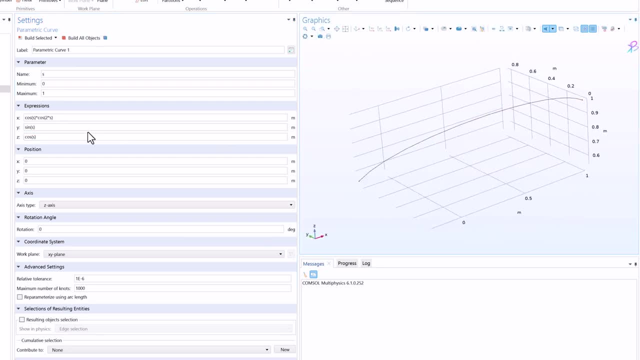 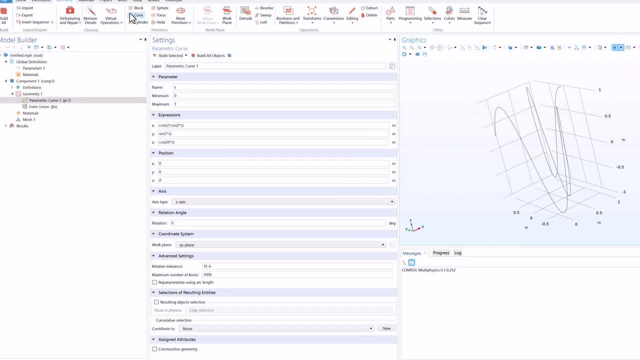 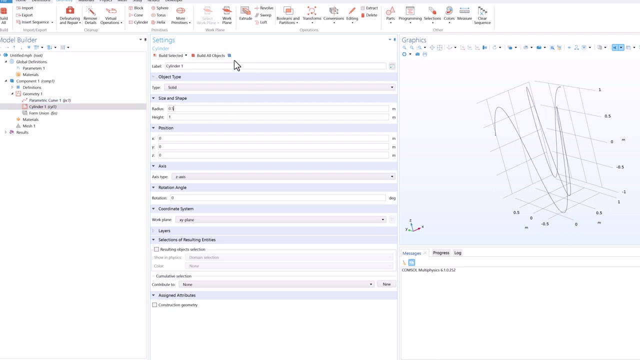 and and we can create these geometries. maybe I'll increase the frequency of y and similarly for z. also I can increase the frequency. and you see that we have a complicated curve in 3d right. so what can you do with this, for example? I'll show you an example for this. so let's say I have a cylinder and the radius is 0.5. 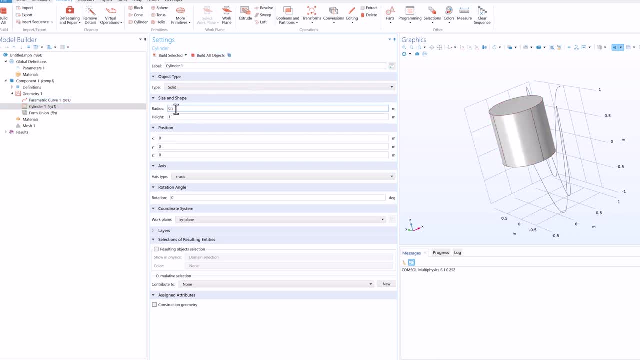 meter and click on build selected. it's too big, so I will write 10 cm. by the way, uh, you can write the unit in the third packets and height. i'll make this one centimeter. okay, so i have this, uh cylinder and the curve. now i'll also make the radius. 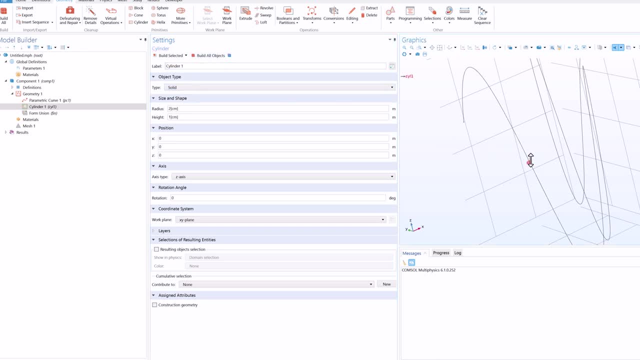 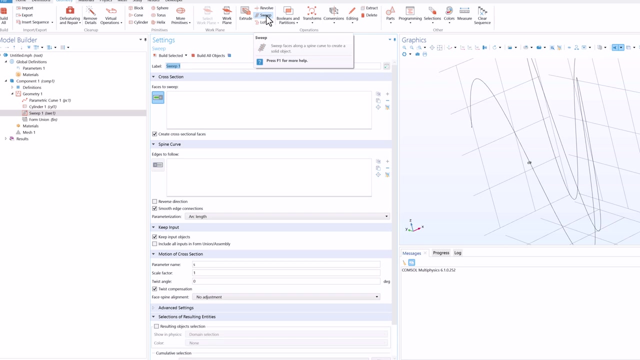 to two centimeter. i think this is fine. so what we'll do now is that we'll click on sweep. so if you keep the cursor here, you will see that it's written: sweep a face along a spline curve to create a solid object. so what we'll do here is that we'll zoom in and select the top. 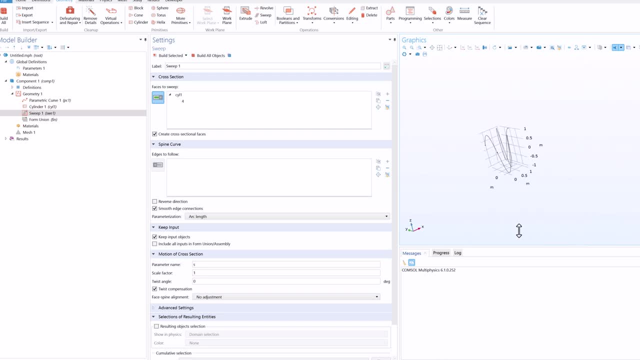 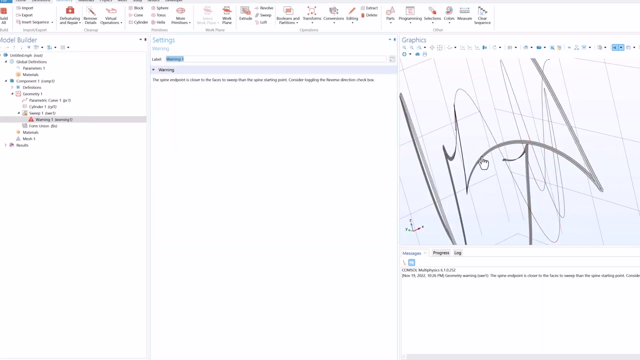 surface to be the face to sweep and in the spline curve. we'll select this curve and we will not touch any of the settings here- and click on build all object and you see that we get a curve which is quite, uh, complicated. so we have to change some settings. 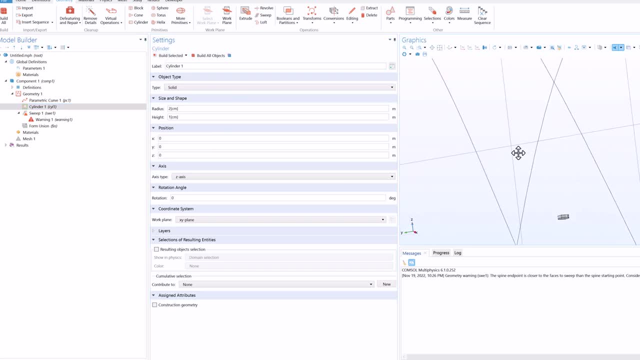 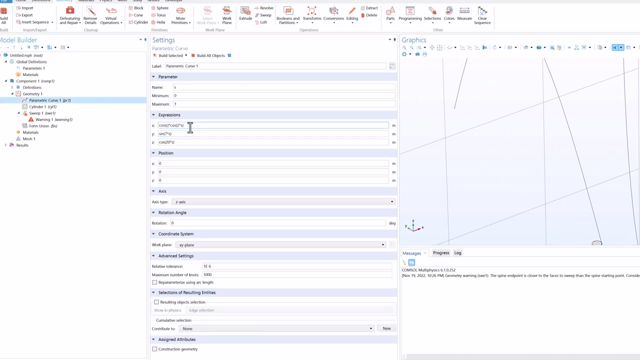 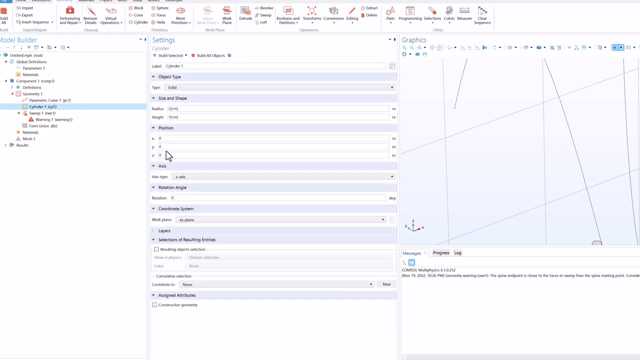 so we click on build selected. now what we will do is we will change the position of the cylinder to the starting point of the curve. so if i go to parametric curve, the value of x is 1, y is 0 and z is 1. so this is 1, 0 and 1 and click on build selected. 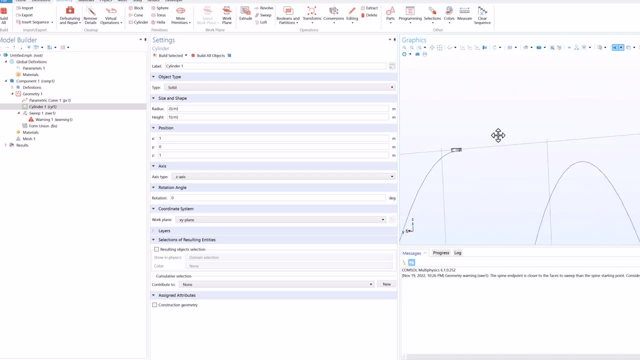 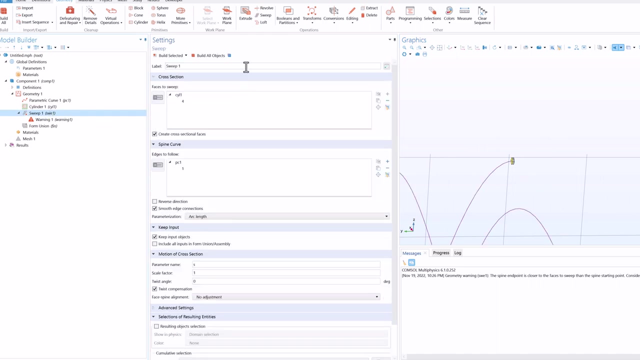 so i have this curve here now in the axis. i'll select y axis. now this looks quite fine now, if i go to sweep again and click on build our object. now you can see that i have a nice geometry. so now i'm going to explain what went wrong in the 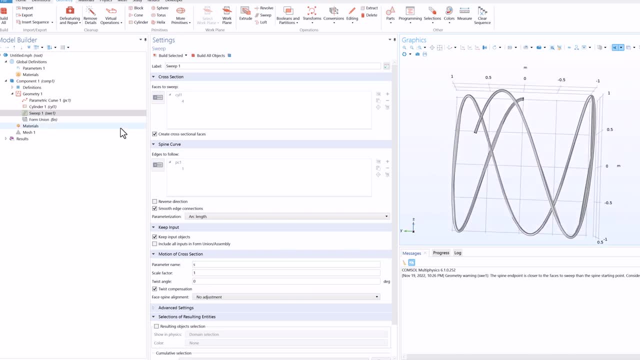 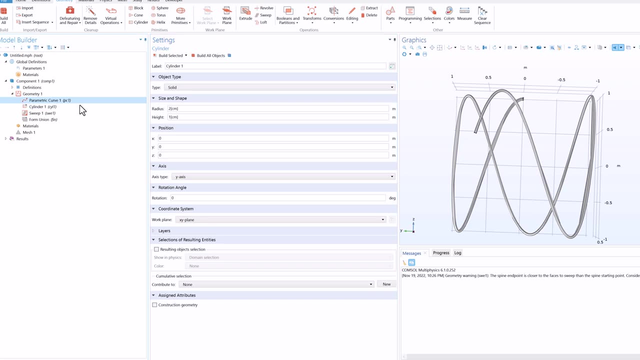 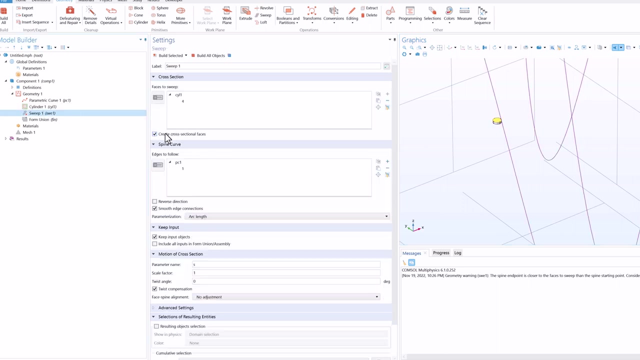 previous uh try, so i'll just change the setting that was before. uh, so this was the initial stuff that we did, and also it was z axis. so this is what we did in the previous case, but we did not get a nice curve. now what is happening here is that when i go on to sweep and select face to sweep as this: 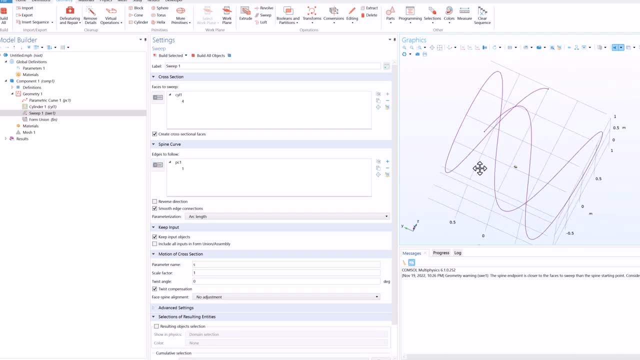 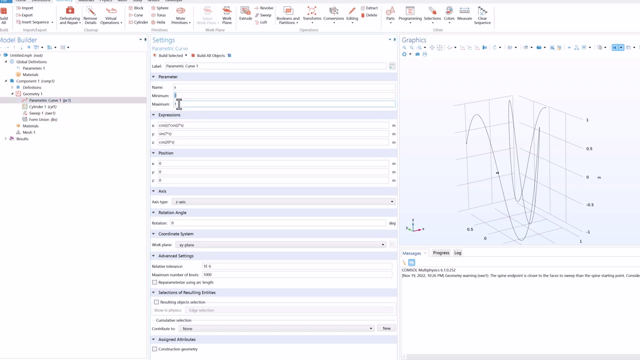 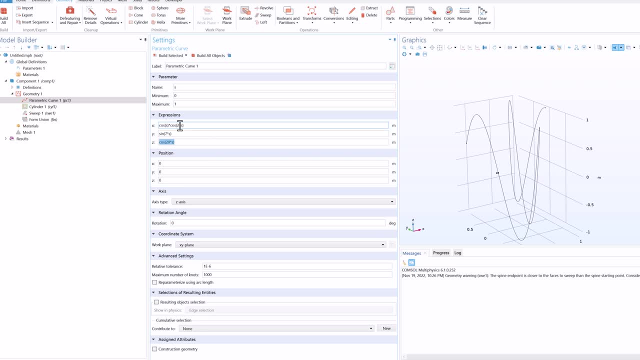 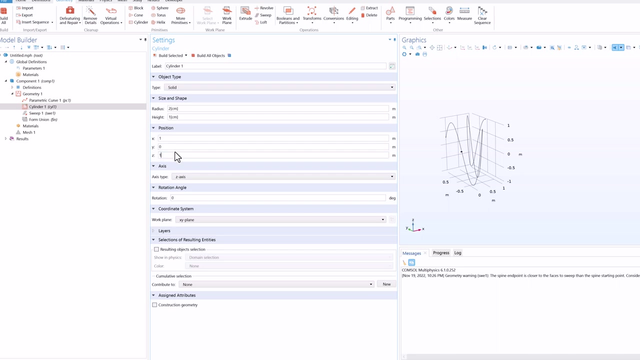 y is 0 and z is 1, so the coordinate is 0. no, sorry, the coordinate is 1, 0 and 1. so basically, this point is 1, 0, 1. so what I did? I went to the cylinder and change the position to 1, 0 and 1 and then click on build selected to position my. 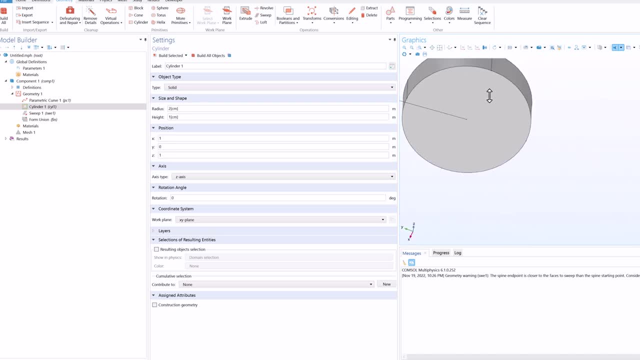 cylinder at the starting point of the curve, as you can see here. right? so after this, I rotated the cylinder along the y-axis to create a cylinder and a path. so this will help the software to follow the curve along with the face, because it is almost perpendicular to the face. right? so after this we go. 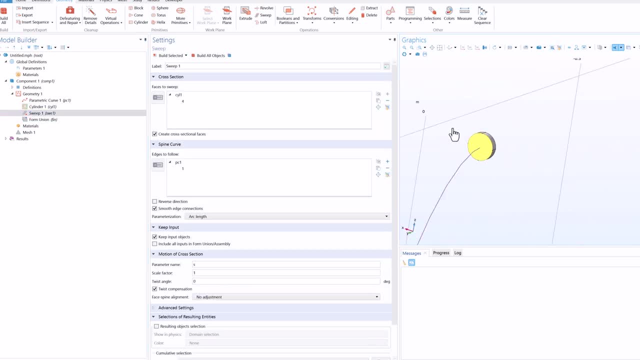 on to sweep and then open up the face to sweep and select the surface and again in the edge to follow select the curve and click on build selected or build selected. then you can automatically move on to complete that. view that video. now you can see you can choose the чего type your action order for a. 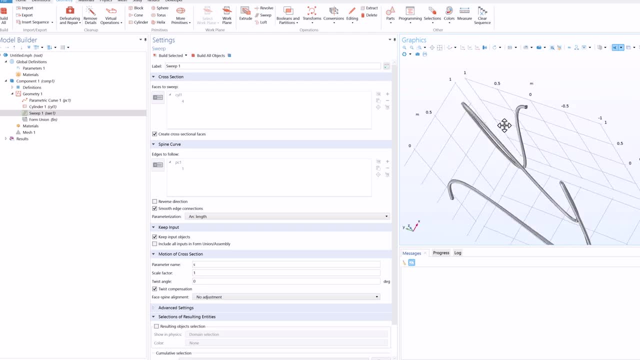 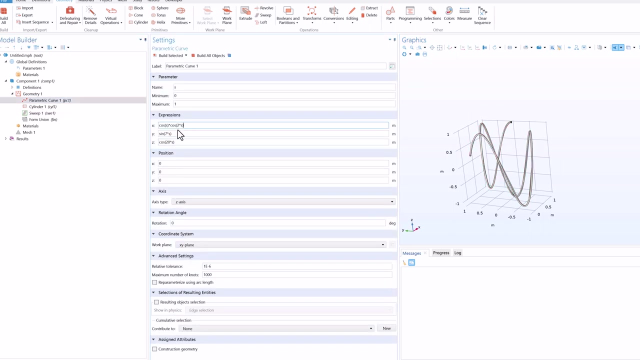 all object doesn't matter, and you will have the required geometry. now, if you try to create this kind of a geometry manually, it's almost impossible to do so. this is really handy. the only thing you have to work is you need to know the equation which follow the particular curve that you need. 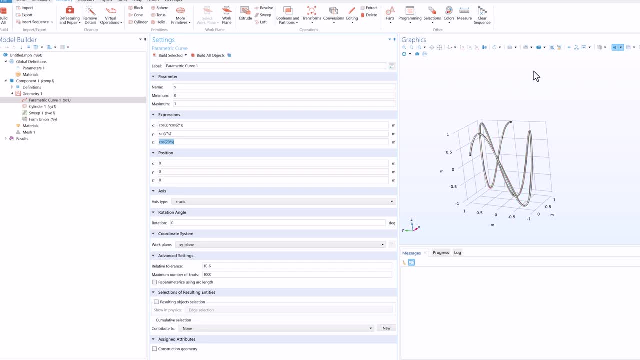 for your project, so i hope, uh, that this tutorial is helpful to you. uh, please do subscribe to this channel because, uh, as per the data, like 90 of the people are not subscribing. so just subscribe, it's free. uh, it helps me to get motivated to create more videos, so, okay, i'll come back to the video. 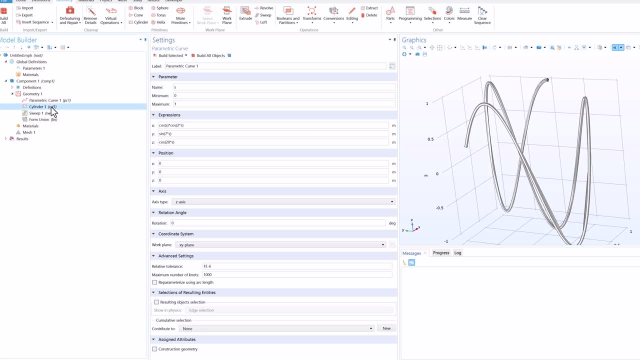 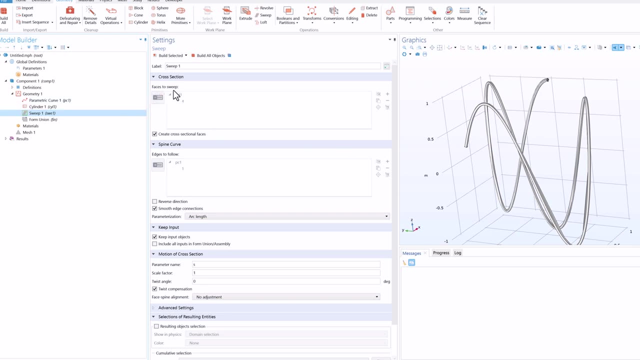 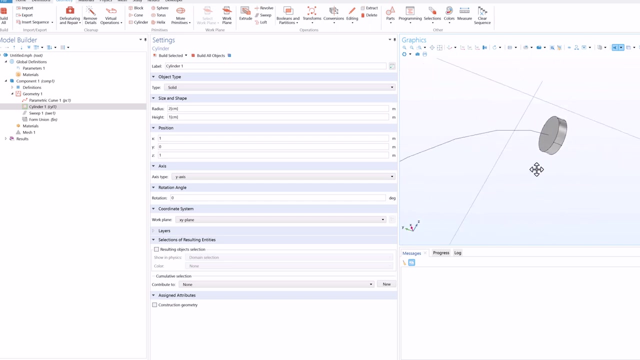 once again. so there are few things which you need to take care when you use the sweep feed feature, that is, uh, when you select a face and the curve that the face is following, make sure that the two objects, that is, the face and the curve, are aligned together. for example, the cylinder. 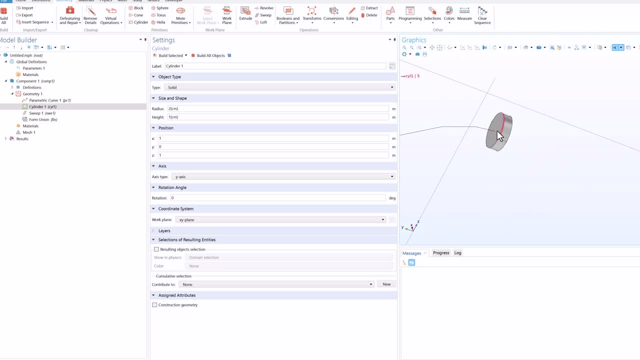 can be placed a bit far away, but it should be aligned. uh, the ideal case it should be permanent, equal to the starting point, so that it can easily follow along. so let's say, if i move the position a bit, for example, i move it along y, so minus 0.1, and click on build selected. so now i have a 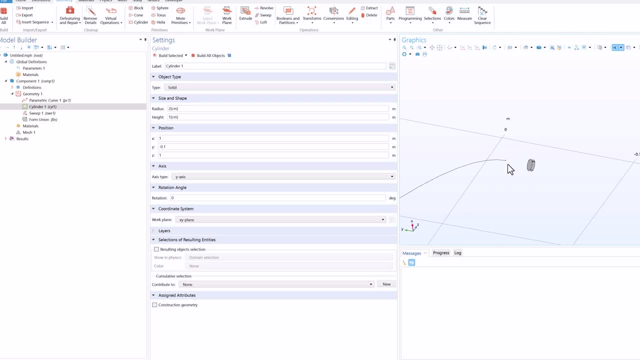 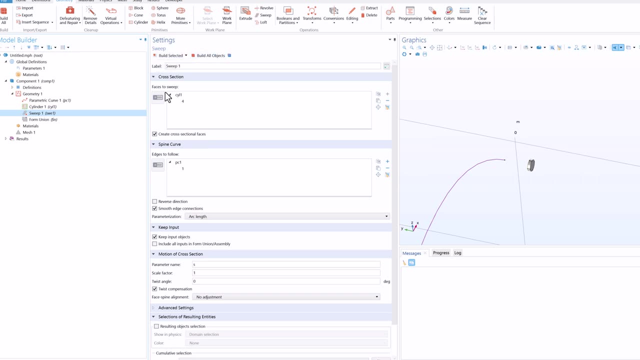 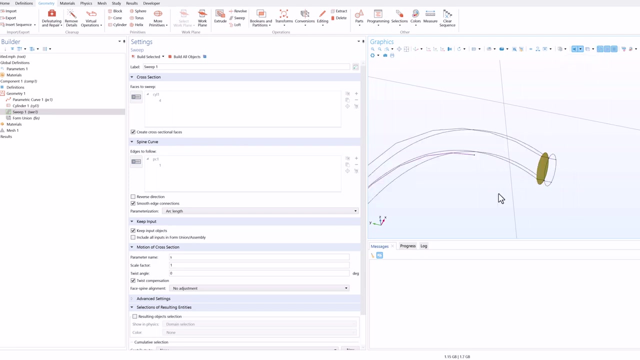 cylinder here, but the curve starts after 0.1 uh meter. now if i go to zip and again do that, so you will see that i have the cylinder, and then it tries to forcefully create the uh parametric curve and the cylinder. so if i click here you see that i have the cylinder here. 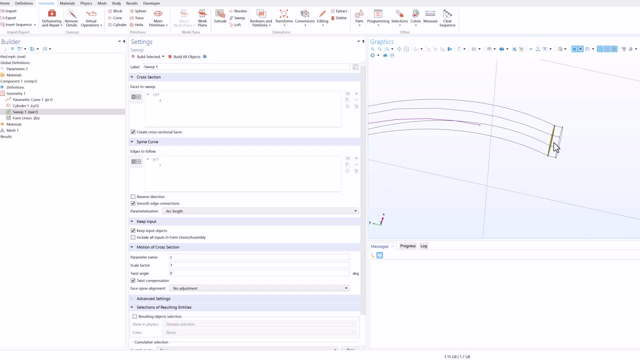 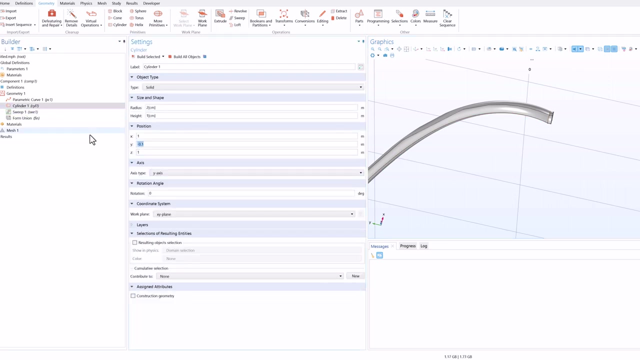 and the parametric curve here, so the software try to forcefully create this solid geometry from the cylinder to the curve. it does not look that great, so that's why I said that the best thing is first you align the curve through which you want to follow the 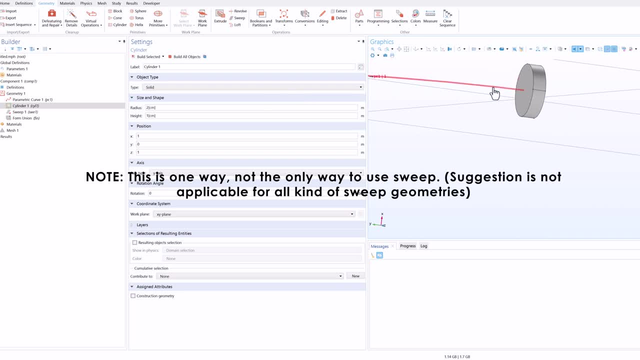 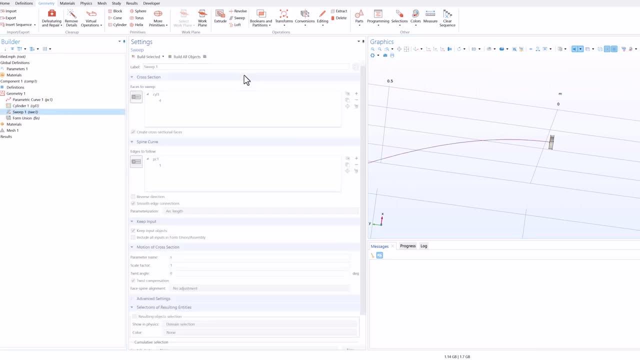 geometry and keep the face perpendicular to the curve or the face that you want to sweep, and then you create the settings for the face and the edge and you will have a nice geometry. and of course you can play with the settings, for example, reverse direction, twist, compensation and so on. those are 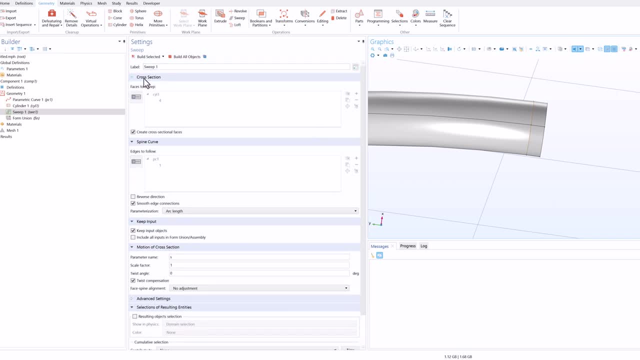 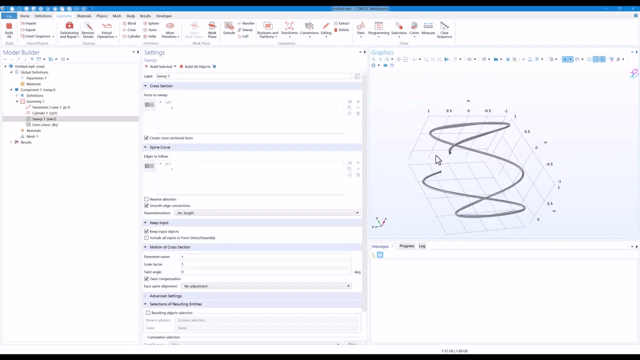 according to the software. It is up to your personal preference depending on the project you are working, but this is the overall idea: how you can create complicated shapes in comsol without using any third-party software or tool. that's it for this video. I hope you found this useful and also you can check out my courses. those are there in. 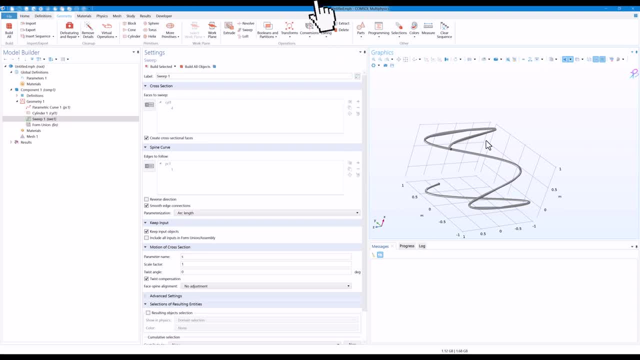 the description. you can check them out. thanks for watching and have a nice day ahead.